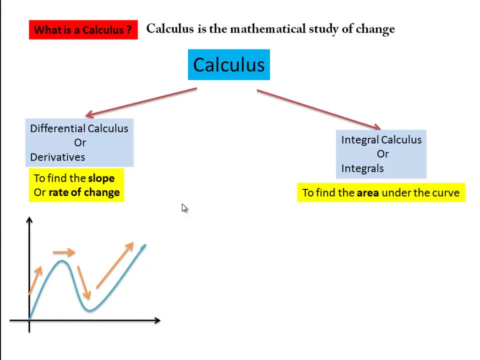 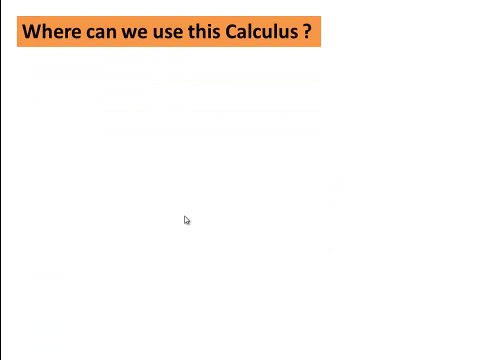 Suppose we have a graph. Differential calculus will help us to find how much the graph is increasing or decreasing. Integral calculus will help us to find the area under the curve. Where can we use this calculus? Calculus has so many great applications in our real life. 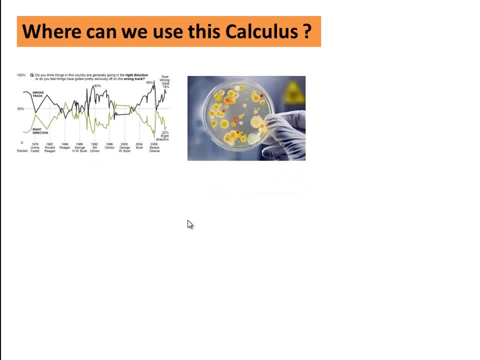 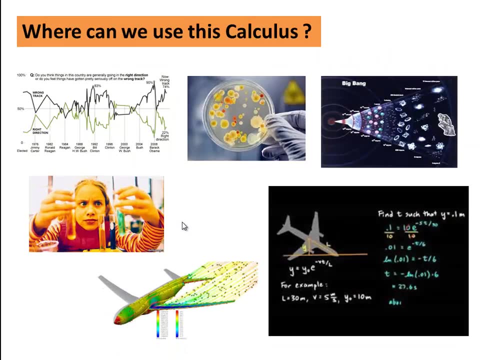 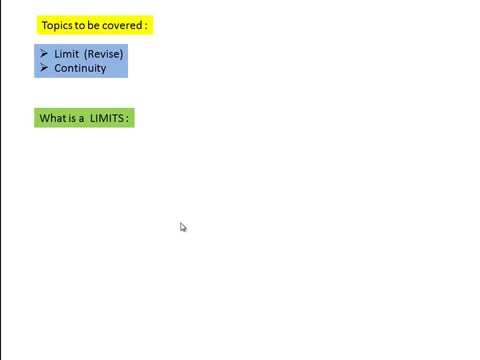 It is used in economics, medical science, astrophysics, chemistry, engineering, Aerodynamics and so on. Now the topic that we are going to cover will be limits and continuity. First, what is the limit? Let us take a function f of x equals to x plus 2.. 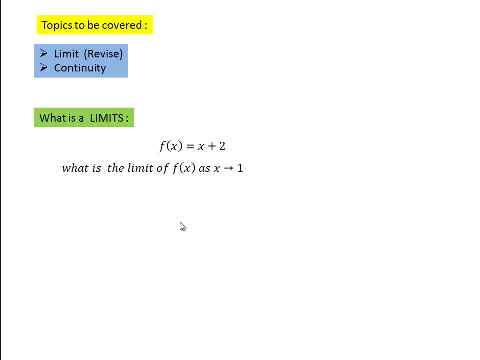 And a question: what is the limit of the function f of x when x is approaching towards 1?? Here we have a table column Now when we take x value, smaller and smaller, very close to 1.. So when we decrease the x value and reaching very close to 1,, 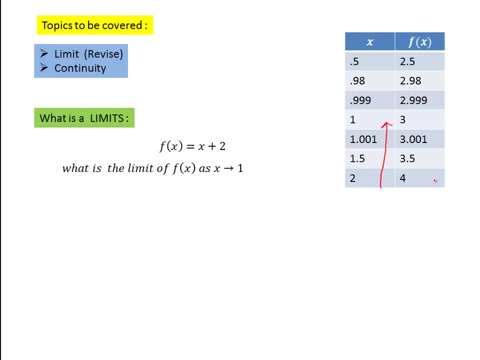 then we notice that the value of f of x is decreasing and decreasing and approaching very, very close to 3.. Now another case when we increase the x value and approaching very, very, very close to 1.. See, we are going to increase the x value and approaching very close to 1.. 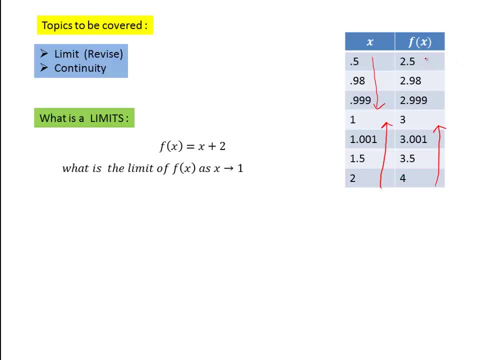 Then again we notice that the f of x value is increasing, increasing, increasing and approaching very, very, very close to 3.. So from either case we observe that when the x value is approaching very close to 1, then the value of the function is approaching very close to 3.. 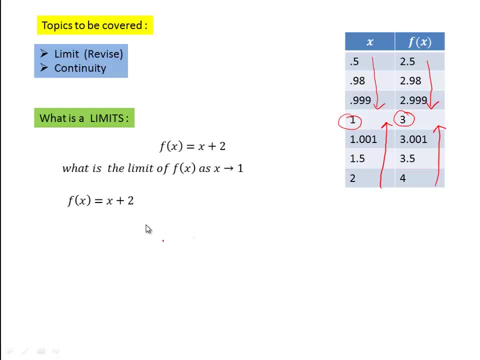 So in this function, f of x equals to x plus 2, when x value is approaching very close to 1,, this value of the function is approaching very close to 3.. Now, this number 3 is nothing but the limit of this function when x is approaching towards 1.. 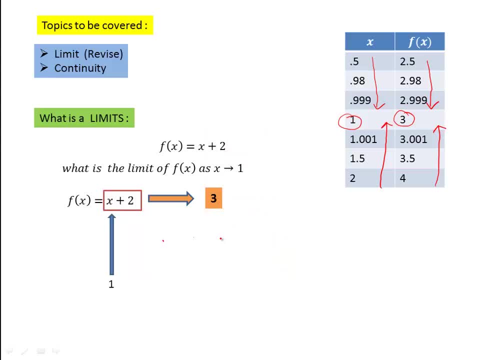 Okay. so how do we write a limit? We write in this way: Limit when x is approaching towards 1, then the function f of x. So limit: x is approaching towards 1, the function f of x. here we have x plus 2.. 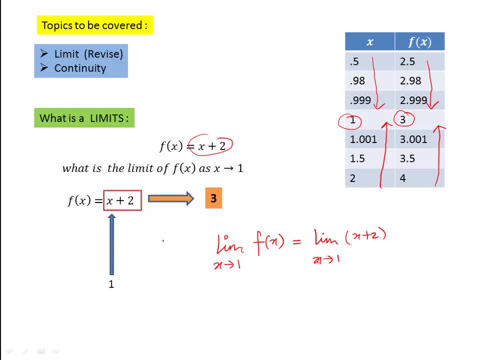 So the limit of x plus 2, when x is approaching very close to 1, is nothing, but in the place where x, we are going to take 1, 1 plus 2 is equals to 3.. So this 3 is the expected value of the function when x is approaching towards 1.. 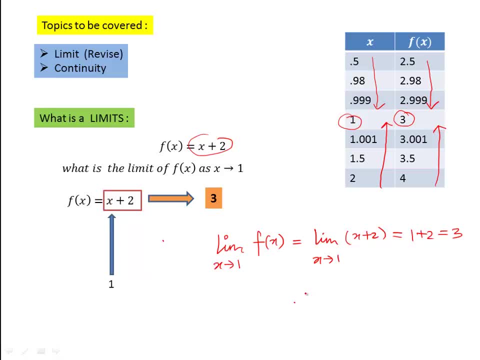 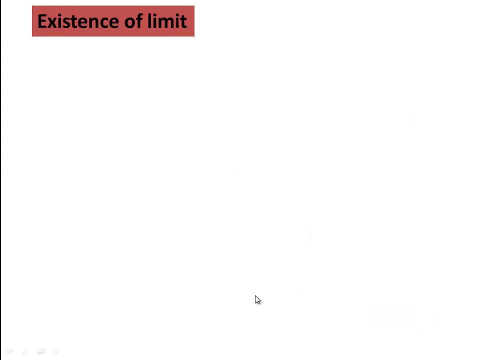 And this is how we write in a limit form. So limit is nothing but the expected value of a function. Now next question is existence of a limit, whether the limit exists at a particular point or not. A limit of the function f of x exists at. x equals to a. 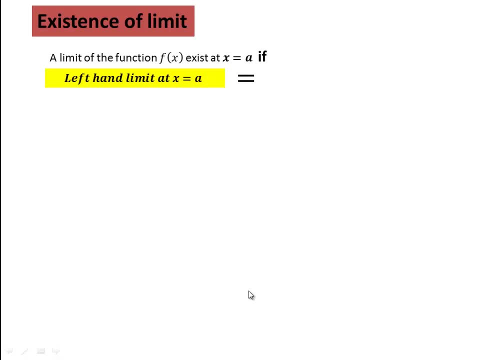 if the left-hand limit at x equals to a is equals to right-hand limit. at x equals to a. If the left-hand limit equals to right-hand limit, then we say that limit exists at that point and the common value is taken as a limit. 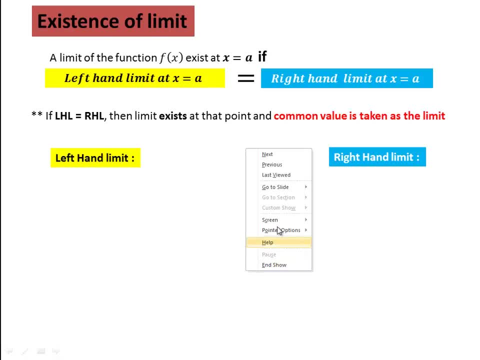 Now, next, how do we write left-hand limit and right-hand limit? So it is similar: Left-hand limit at x equals to a. we are going to write as a limit x tends to a and we write negative of f, of x. 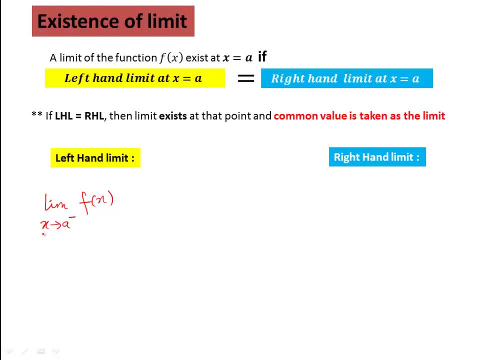 This negative denotes that x is approaching towards a from the left. So this is how we write for left-hand limit And right-hand limit. we write: x tends to a plus f of x. Now this indicates that x is approaching towards a and plus indicates that x is approaching towards a from the right. 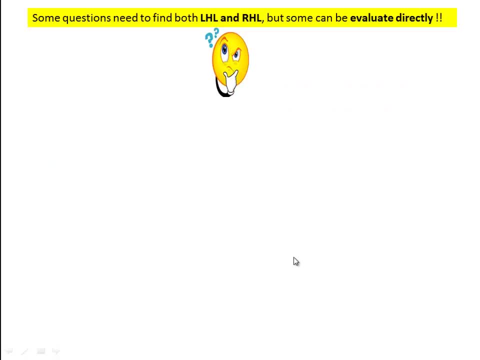 So this is how we write: left-hand limit and right-hand limit. Now some questions: we need to find both left-hand limit and right-hand limit, But some questions can be evaluated directly. Now the question is: how can we distinguish? 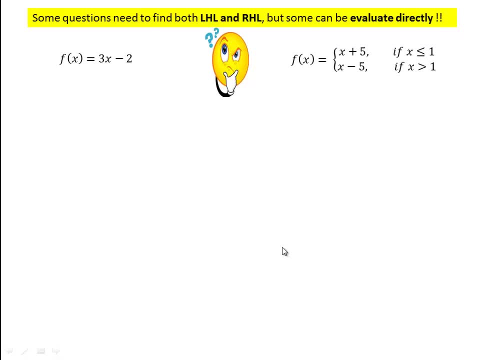 So I have given two functions, one on the left and one on the right. So the question is: what is the limit of f of x as x is approaching towards 1?? Now, approaching towards 1 means we have two cases. 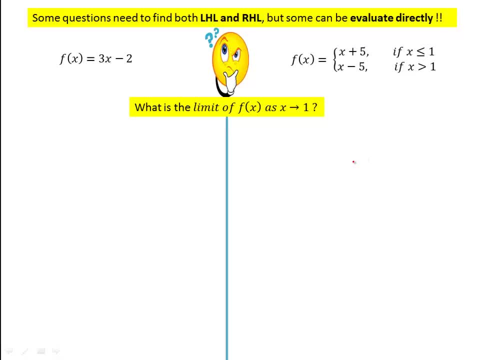 One is approaching towards 1 from the right, One is approaching towards 1 from the left. So when x is very, very, very, very close to 1, means we have two cases, slightly greater than 1 and slightly less than 1.. 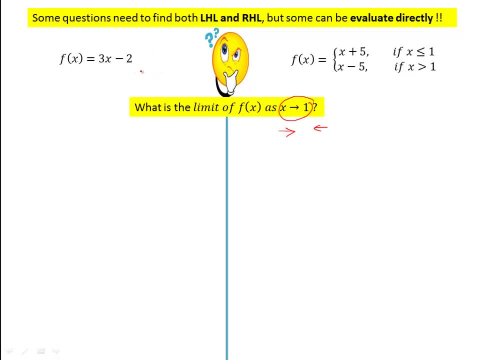 So in the functions on the left-hand side, when x value is taking slightly less than 1, again we are going to take this function. When x value is slightly greater than 1, again we can take the same function: 3x minus 2.. 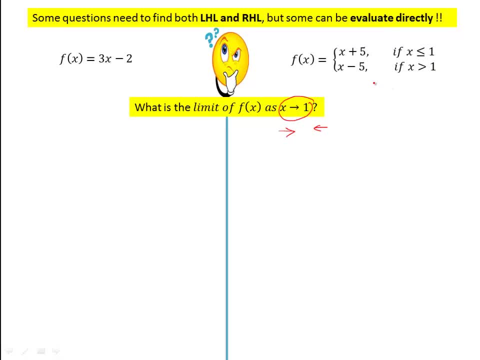 But on the right side. when x value is slightly greater than 1, we need to take this value, x minus 5.. When x value is slightly less than 1, we need to take this value, x plus 5.. So when x is very close to 1,. 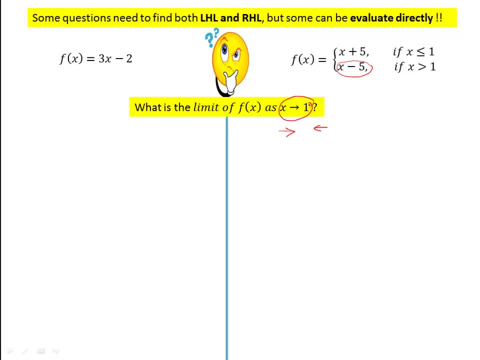 we have two cases, slightly greater than 1 and slightly less than 1, for this particular question. So we have to take two different values of the function. So for this kind of a function we need to use left-hand limit and right-hand limit. 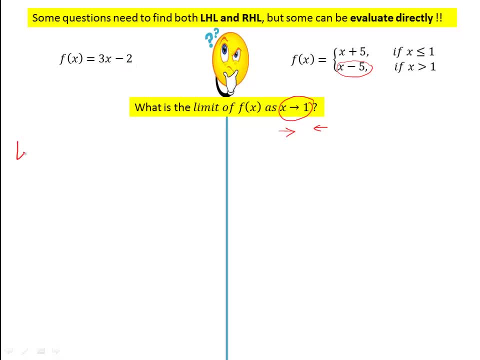 This one we can find directly. So this will be limit. x tends to 1,. f of x is equals to limit. x tends to 1, 3x minus 2 equals to 3, 1 equals to 1.. So this will be the limit of the function on the left. 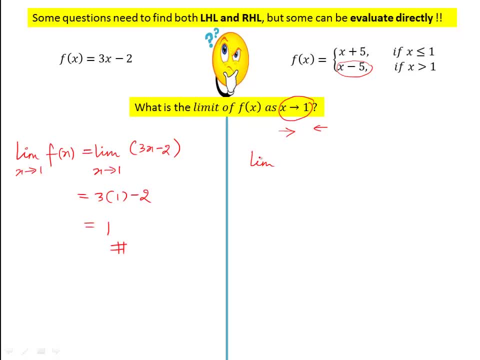 Now the limit on the right. So when x is very close to 1 from the left, so we are going to write negative. In this we are finding left-hand limit, So limit x tends to 1, negative. 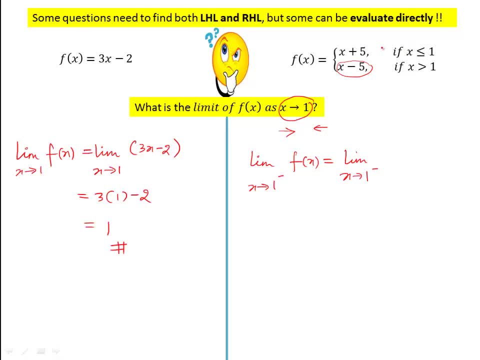 That means very close to 1. from the left means we need to take this function right: x plus 5.. So the limit will be in the place of x, we are going to write 1.. So 1 plus 5.. 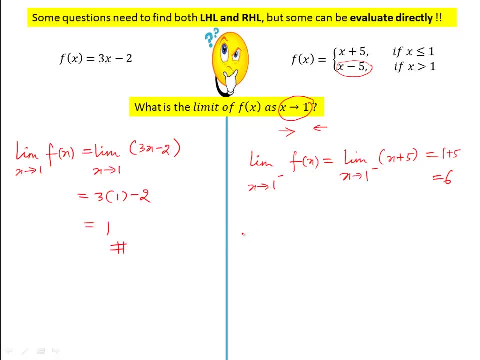 is equals to 6.. Now next is when x value is approaching towards 1, from the right means, slightly greater than 1.. So when x value is slightly greater than 1, we need to take this function: x minus 5.. 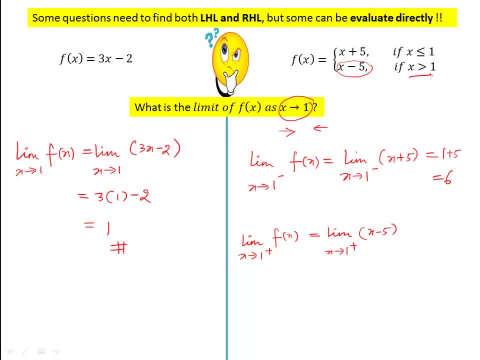 So x minus 5, because the condition is written here. When x value is greater than 1, we need to take this function. When x value is less than or equals to 1, we need to take this function. So condition is already written on the right side. 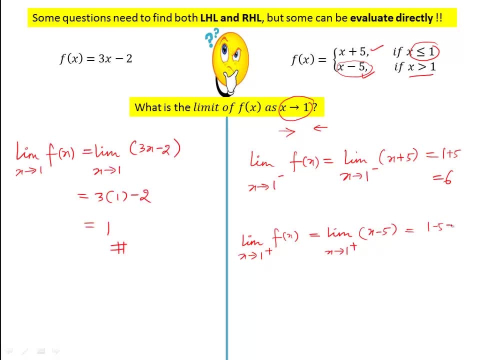 So this will be: 1 minus 5 equals to negative 4.. Now we can observe that left-hand limit is 6 and right-hand limit is negative 4. So left-hand limit is not equals to right-hand limit. Therefore we can say that. 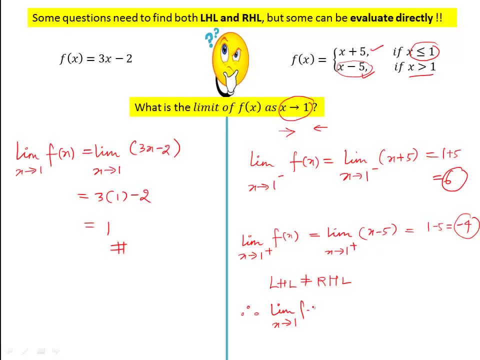 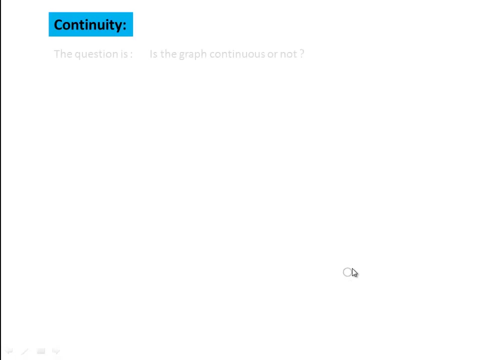 limit x tends to 1 of f does not exist. This is how we find limit at a particular point. Okay next, The next topic is continuity. The question is: is the graph continuous or not? So we will be given a graph. 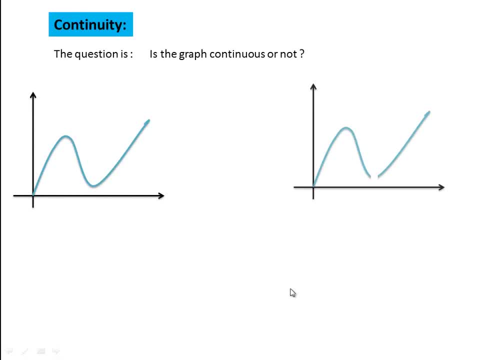 We are going to say whether the graph is continuous or not. So I have two graphs, one on the left and one on the right. Now, which one do you think is a continuous graph? Yes, very good, This one is continuous. 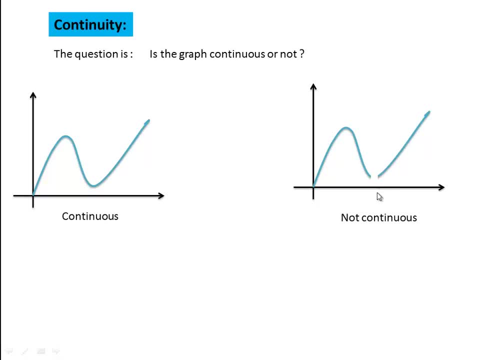 On the left is continuous. on the right is not continuous because we see a break in the right-hand side graph right. So normally graphically we can say that the graph is continuous if we can draw the graph Without lifting the pen from the plane of it. 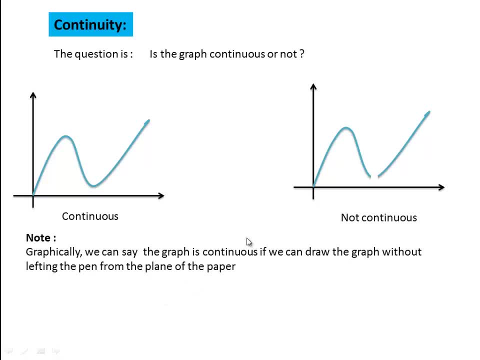 So it is easy to judge. If we are able to draw a graph without lifting the pen, then that graph will be continuous. Let's say x will do some a, So when x equals to a and there is no y value, 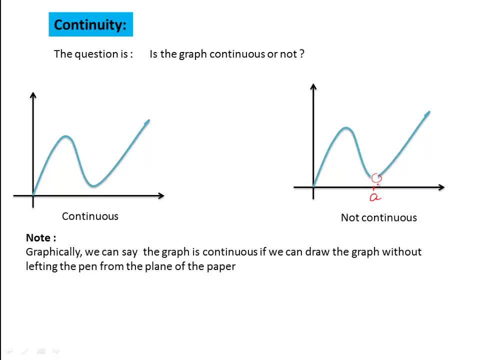 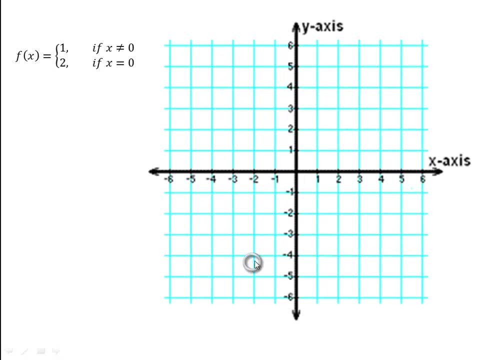 So this function is not continuous at this particular point a. Okay, Now we have a question. f of x equals to 1 when x is not equal to 0.. f of x value equals to 2 when x equals to 0. 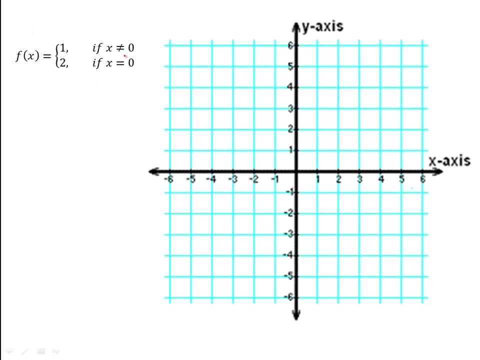 Now we are going to decide whether this function is a continuous or not. This we can easily decide by simply plotting a graph. Okay, we can plot When x is not equal to 0, we are going to take f of x. 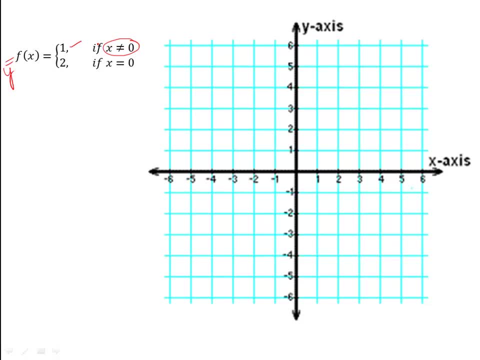 f of x is nothing but y value, right? So when x is not equal to 0, y value is always 1.. So this one x value is negative 1.. x value is negative 5.. y value is 1.. 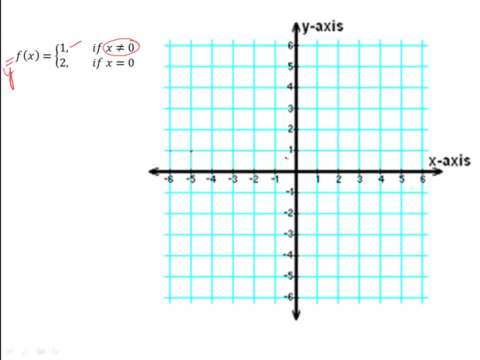 x value is negative: 2.. y value is 1.. All this, x is not equal to 0, right? So when x is not equal to 0, we are getting y is equal to 1.. But when x equals to 0. 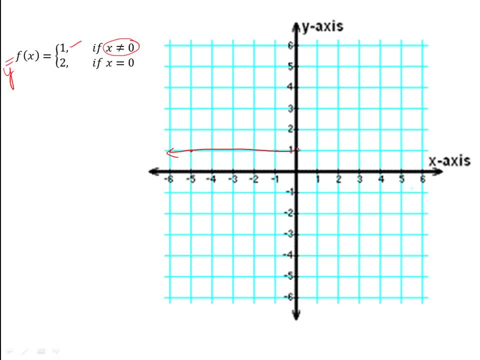 Okay, we are going to write empty. So when x is again increasing, increasing which is not equal to 0. Again we are getting y equals to 1.. Now, when x equals to 0, then the y value is taking as 2.. 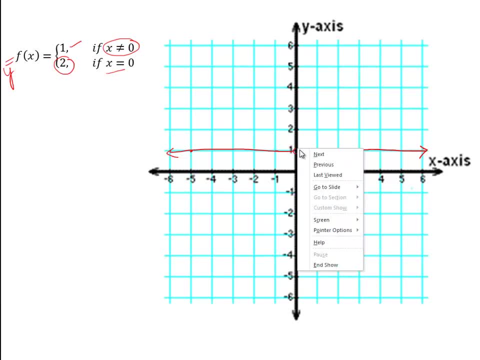 So when x equals to 0, there will be a hole right. So when x equals to 0, y value is taking as 2.. Now we observe that in order to plot this, The graph of this function, we have to lift our pen right. 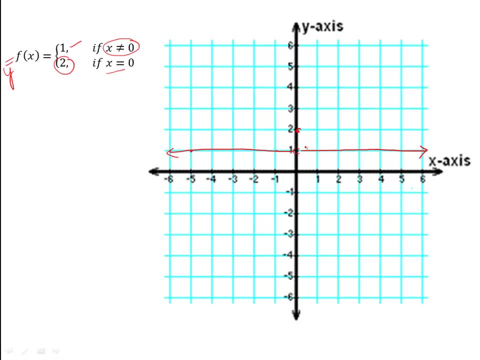 So this function is not continuous. Not continuous at where At x equals to 0. So we can say that f of x is not continuous at x equals to 0. So at x equals to 0, we need to lift our pen right. 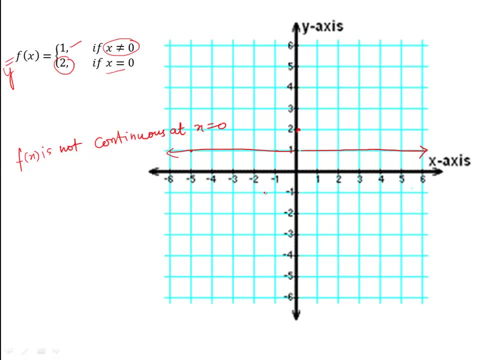 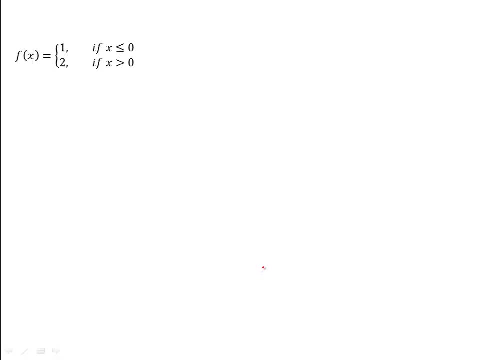 This function is not continuous. at x equals to 0.. Okay, let me take another example. So f of x equals to 1 when x is less than or equals to 0.. f of x equals to 2 when x value is greater than 0. 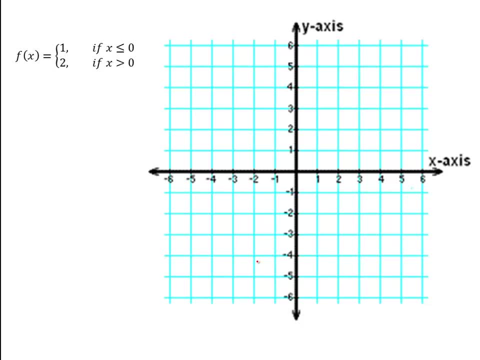 Again, we are going to conclude without this function. So whether this function is continuous or not Now. so here, f of x means it is a y. right Now we see that the y value is taking as 1 when x is less than or equals to 0.. 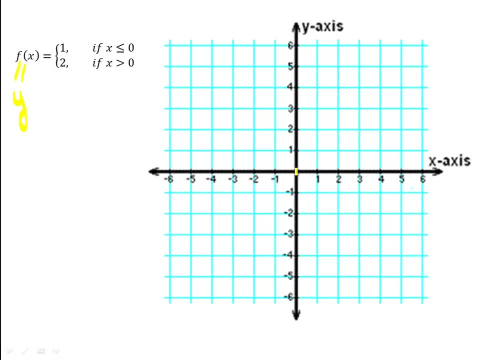 So less than or equals to 0,. all this right From here, it is our x value. From this origin and to the left, everything will be. the x value will be less than or equals to 0.. From origin to the left, y value is always 1, right. 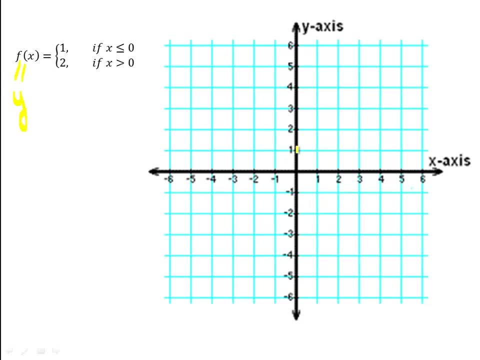 So we are going to take y value And when x equals, when x is greater than 0, then y value is taking as 2.. So when x value is slightly greater than 2, drastically it jumps up and y value is taking as 2.. 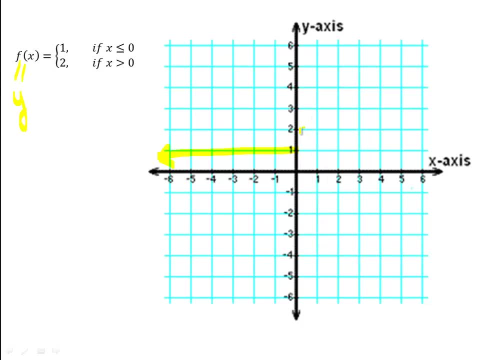 Okay, Okay, Okay, Okay, Okay, Okay, Okay. Now this part. We say that when x value is 0,, y value is 1. And when x value is 0,. right, So there will be a hole here. 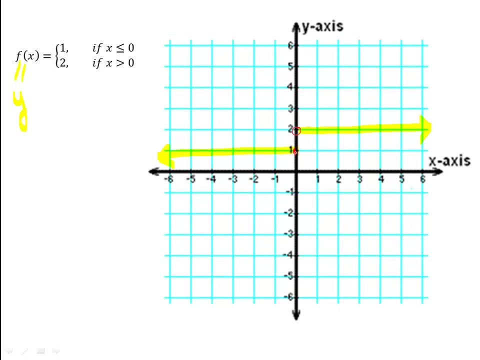 So when x value is less than or equals to 0, then y value is always 1.. When x value is greater than 0, then y value is taking as 2.. So here we need to draw a circle. When x equals 0, y value is not 2, it's 1, right, So it's empty. So we need to draw a circle here. But when x is slightly greater than 0, then y value is 2.. So from here to here, 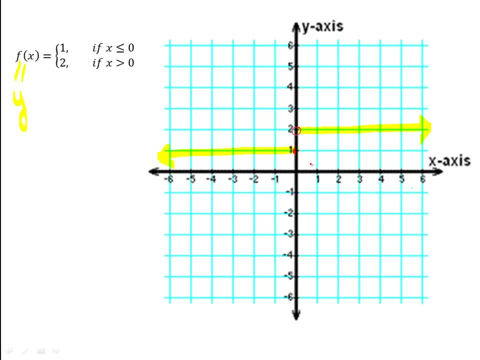 Now again, in order to draw this curve, we have to lift our pen right. So this function is again not continuous, but not continuous at which point x equals 0, right, So f of x is not continuous at x equals to 0.. 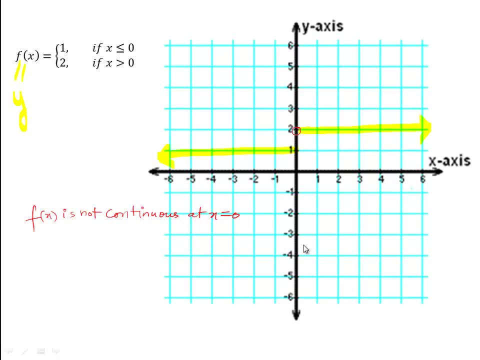 So far these two equations. we have approved, whether the function is continuous or not, By simply drawing the graph. And next time we can solve or we can answer whether the function is continuous or not by not plotting graph, by calculating. So that's how can we do, It's easy. 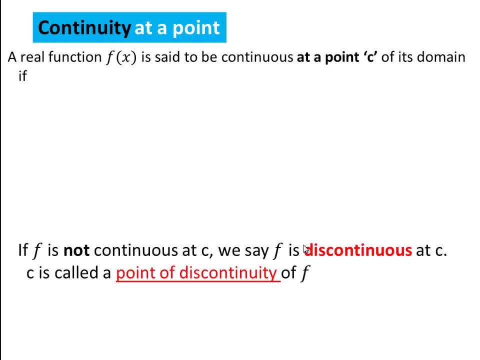 Now continuity at a point A real function f of x is said to be continuous at x at some point c of its domain, If, If the limit x tends to c of f of x exists, So the first and foremost condition is limit should exist at the point c. 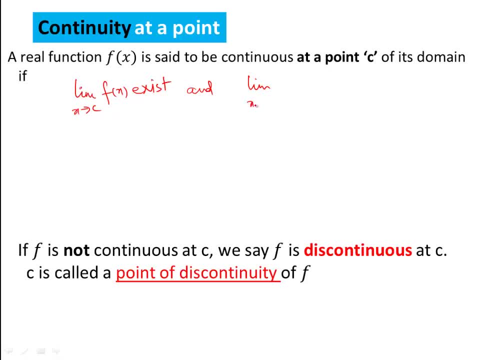 And this limit at f of x, Limit of f of x when x tends to c, should be equals to f of c. So this, So these are the two very important conditions, So a real function. f of x is said to be continuous at the point c of its domain. 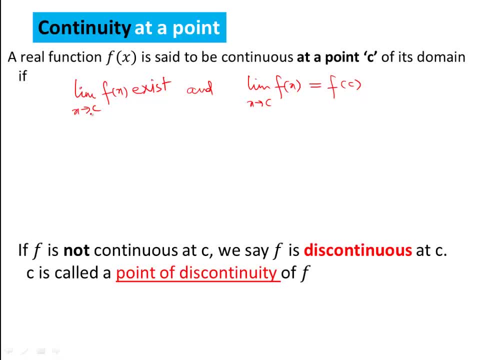 If the limit of f of x- at x tends to c- exists And this value, the value of this limit- should be equal to the f of c, Then we say that function is continuous at point c. Now the question: How can we say that? 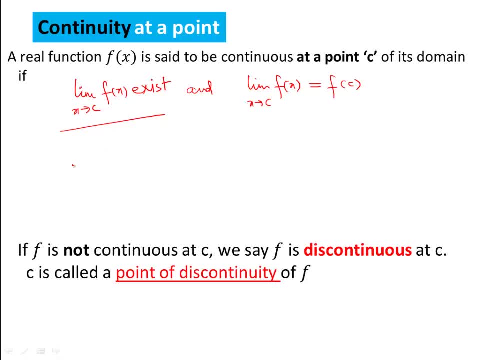 The limit exists at the point c. That one is very easy. We are going to find limit x tends to c, Left hand limit at point c of the f of x, And then right hand limit of f of x at point c, And if we get this value as a same, 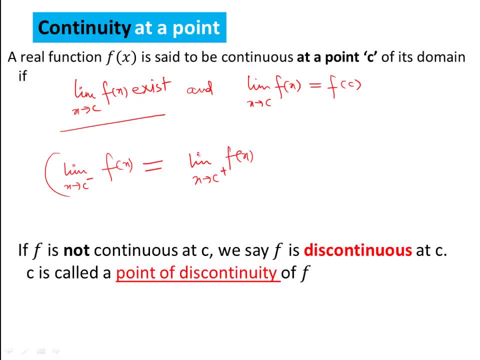 If the left hand limit value is equals to right hand limit, Then we can say that the limit exists And the value this common value is taking as the value or limit of the function Right. And this limit of the function should be equals to f of c.